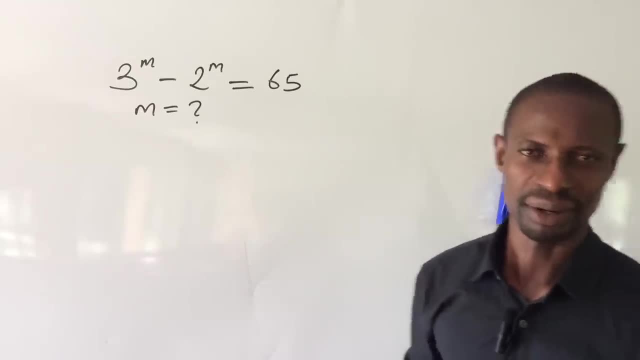 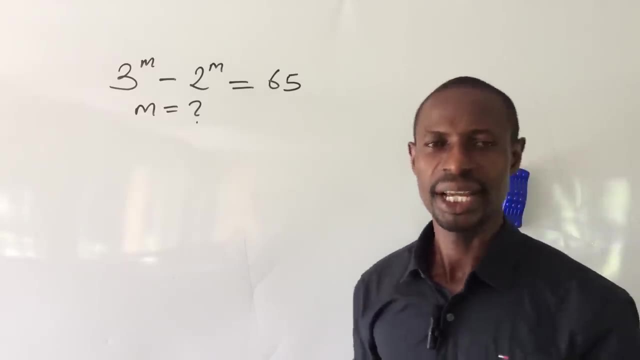 welcome everyone to my channel. today we have a challenge on the board. it's math only paid challenge. math only paid question. so how do we solve this? but before then, uh, if you're new to this channel, kindly subscribe, and when you subscribe, turn on the bell notification button. 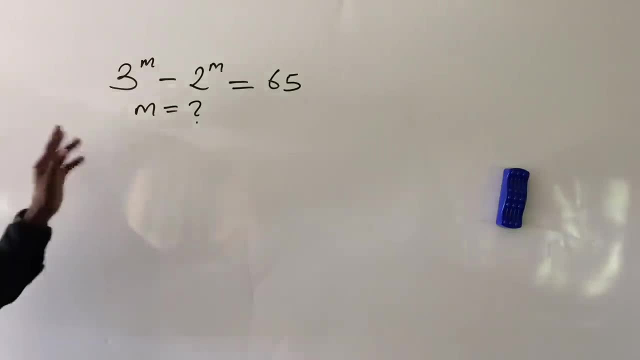 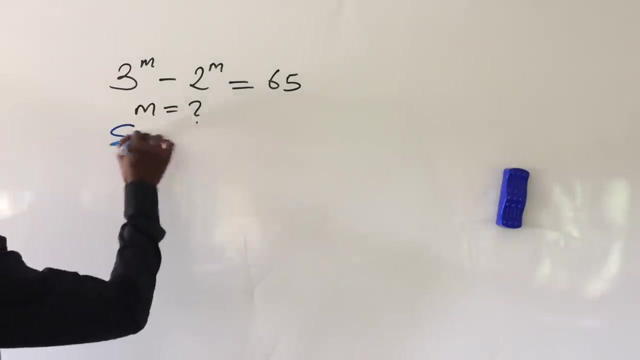 okay, so let's take a look at this question for the day. the question says: three: to the power of m minus 2, to the power of m equal to 65, what there will be the possible value of m. okay, without much waste of time, let's take our question and put down the solution. let's put down the question. 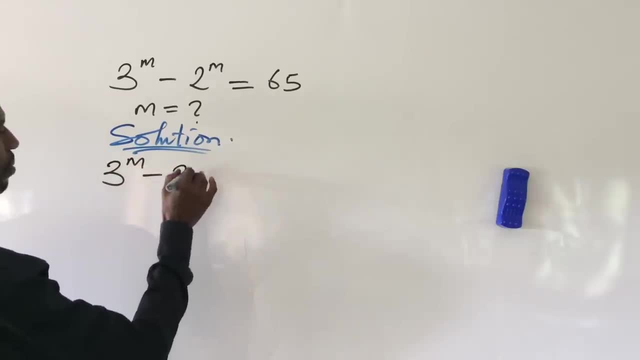 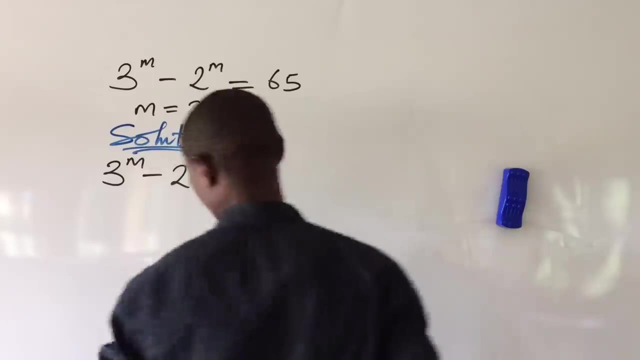 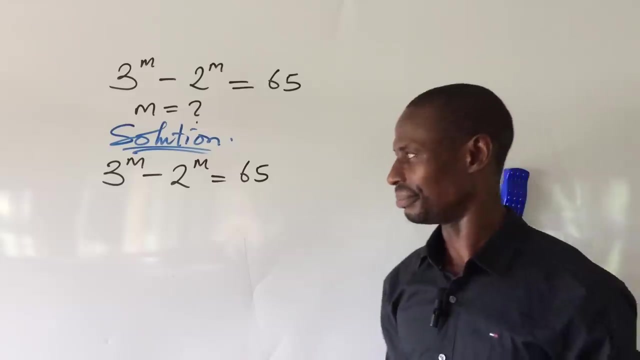 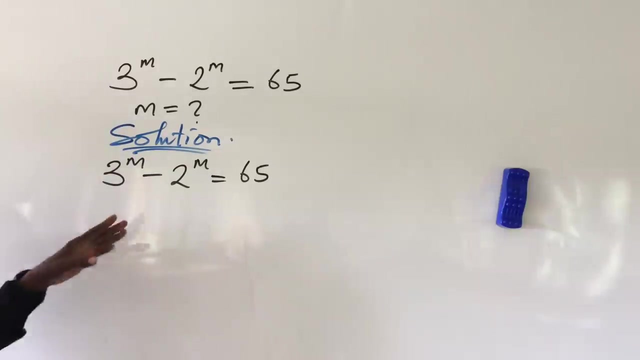 which is 3 to the power of m minus 2 to the power of m, equal to 65. okay now, if you look at this question carefully, this may pose some challenge, but uh, we'll get to solve it with the um knowledge of mathematics we gained in the previous classes. all right, so how do we handle this challenge? it is easy. what we 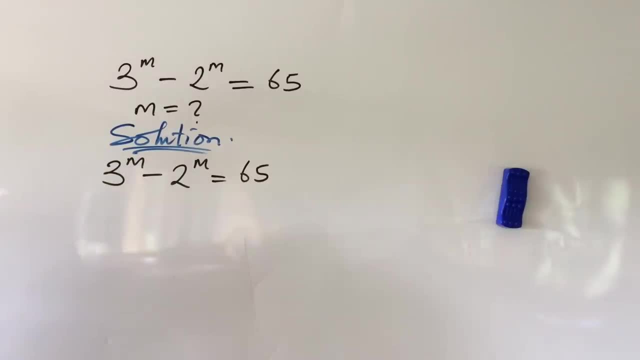 want to do here is to see how we can bring in um another alphabet. but before we can bring in another alphabet in here, we must either deal with the exponents or deal with the base. okay, but here let's handle the exponents. exponents: if I decide to square this exponent, or if I decide to square. 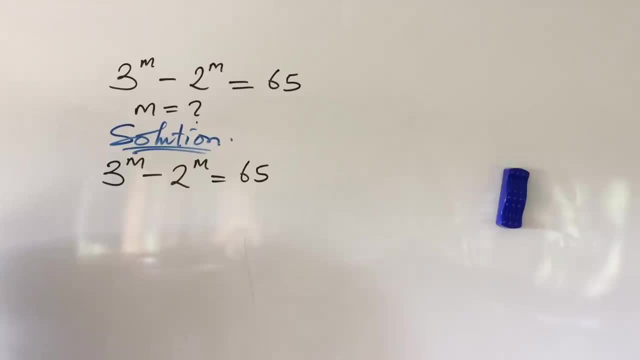 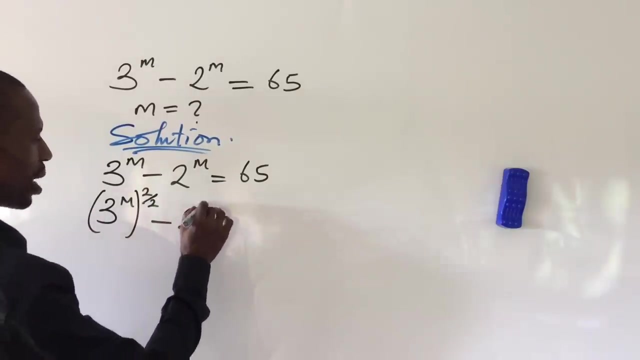 everything here. square everything here. it means I must also square this. so I want to introduce the square without introducing square to this other side, and so I can rewrite this expression here as your: 3 to the power of M R to the power of 2 all over 2 minus 2 to the power of M R to the power of 2 all. 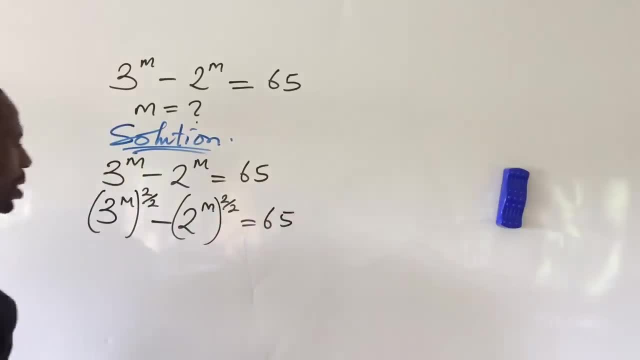 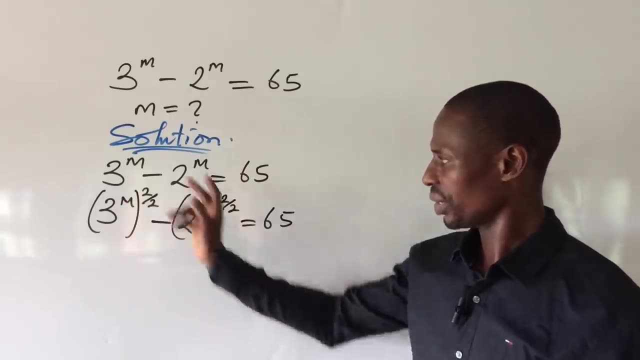 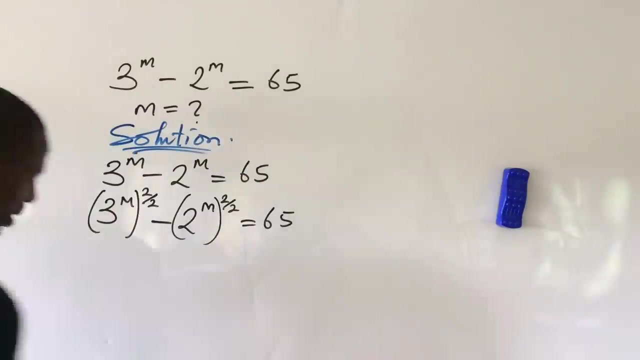 over 2, equal to 65. now take a look at this. here we're having 2 all over 2. we give us 1, then 1 times M will give us M. so 3 to the power of M is still the same thing as whatever we have here. all right, so let's go up to the law of. 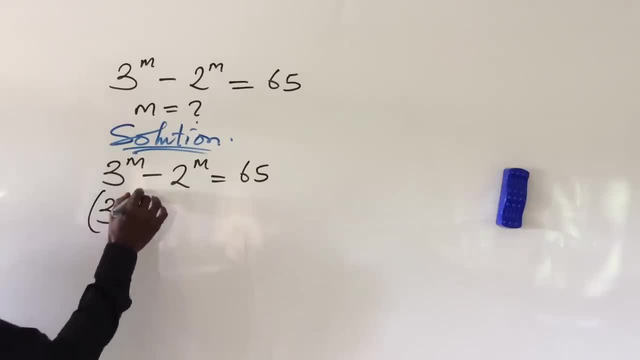 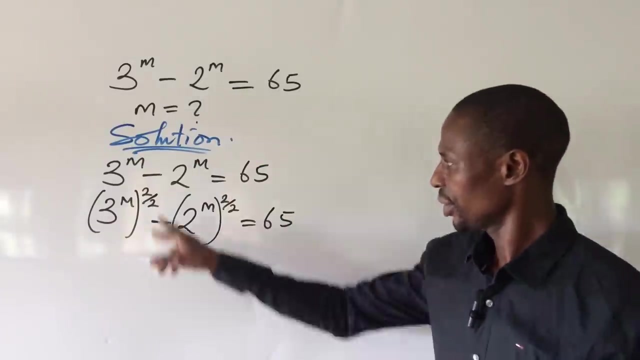 power of m r to the power of 2. all over 2, minus 2 to the power of m r to the power of 2, all over 2 equals to 65.. now take a look at this. here we're having 2 all over 2. we give us 1. then 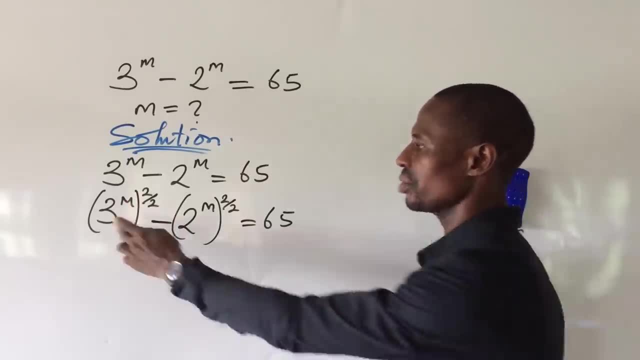 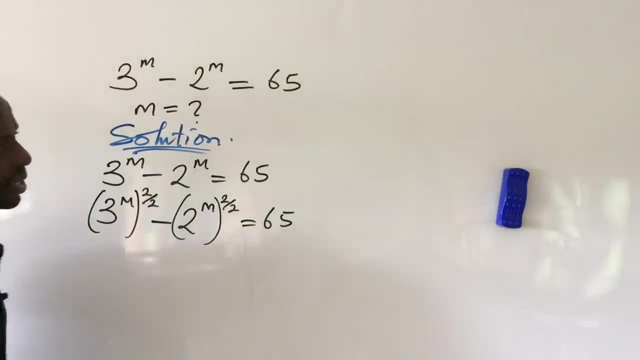 1 times m will give us m. so 3 to the power of m is still the same thing as whatever we have here. all right, so let's go up to. the law of indices says that if you have something, an expression of this kind, that you have a to the power of m. 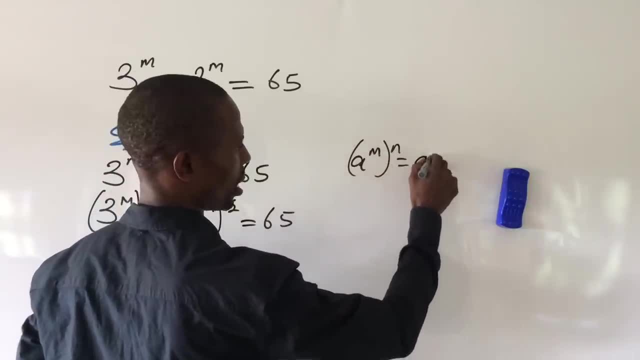 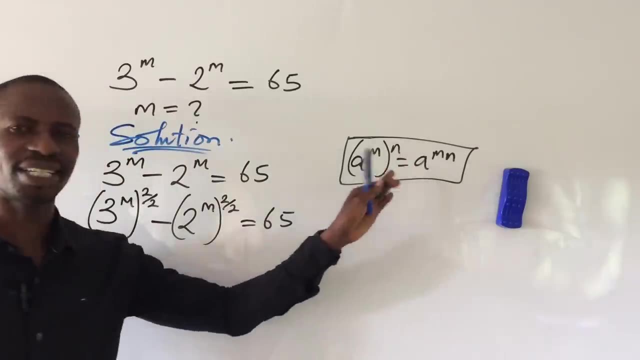 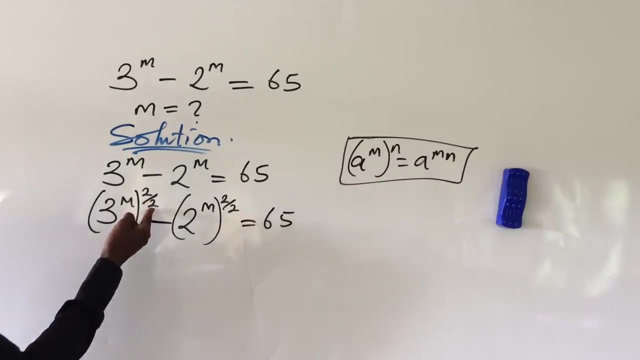 or to the power of n. this is equal to a to the power of m n. okay, in some of our videos we talked about this law in many occasions. okay, so if we suck up to this law, we can bring in this fraction here, we can bring in this fracture here also, and so we can rewrite. 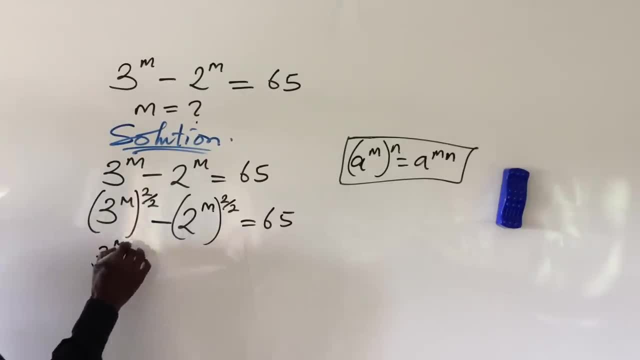 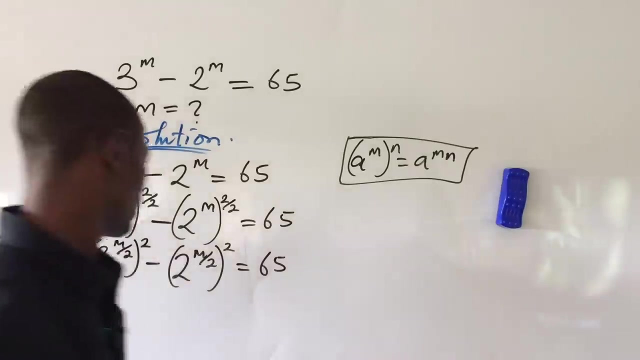 this: your 3 to the power of your m all over 2. close bracket: all to the power of 2 minus 70. we have here m all over 2. all to the power of 2, equal to 65, easy, okay. so we now have a square. here we have. 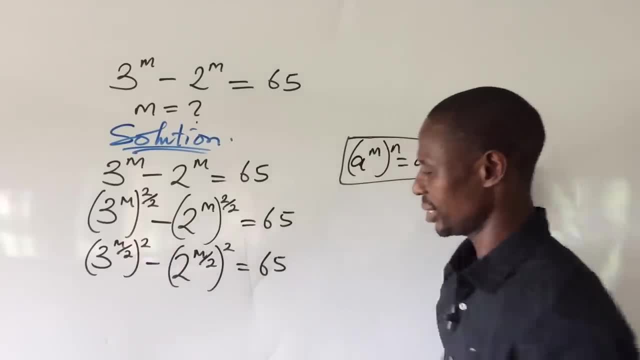 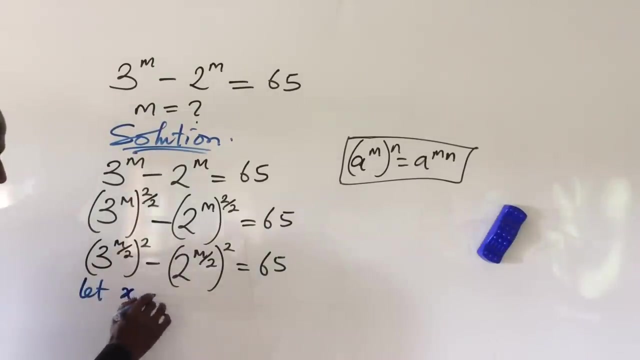 a square so we can bring in different letters to represent what we have in the bracket here and what we have in the bracket here, because what we have in here and here are different so we are bringing different letters. so we cannot say here, let's take x, be equal to our 3, to the power of m. 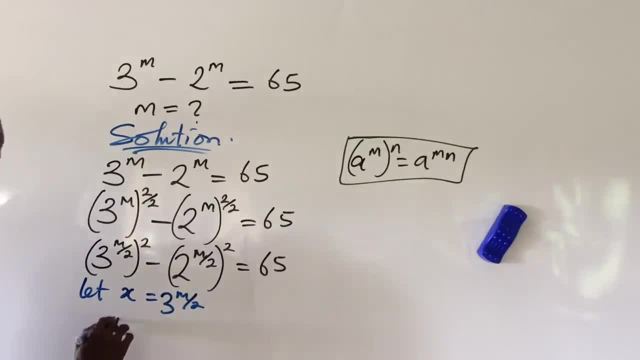 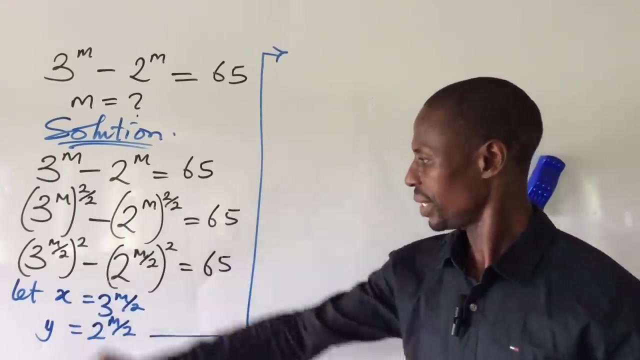 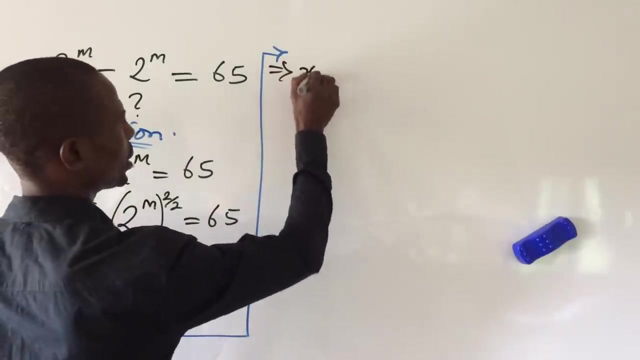 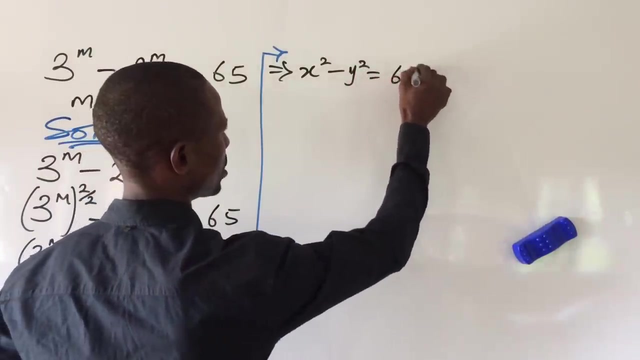 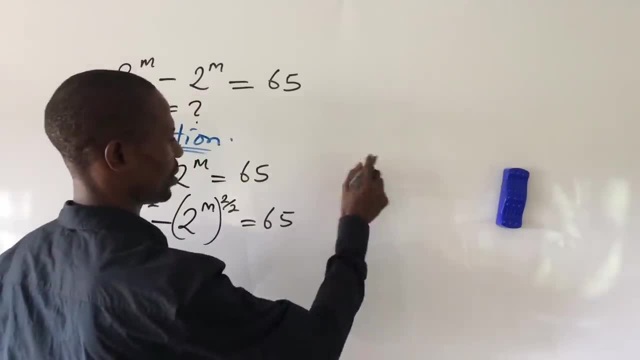 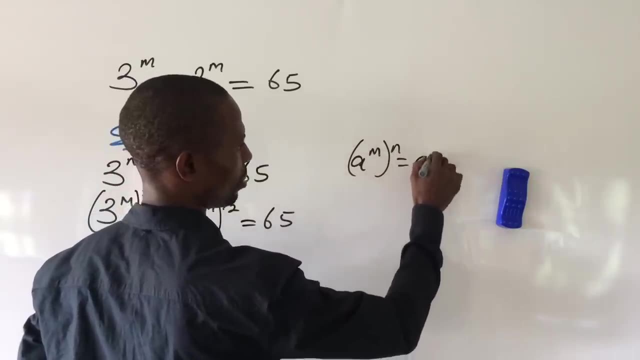 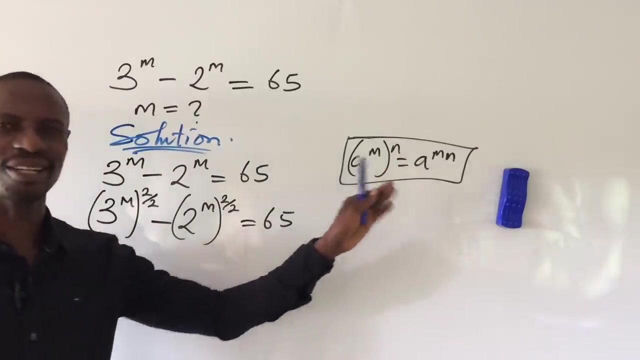 indices which says that if you have something, an expression of this kind in our job, 8 to the power of M R to the power of n, this is equal to 8 to the power of M N. okay, in some of our videos we talked about this law in many. 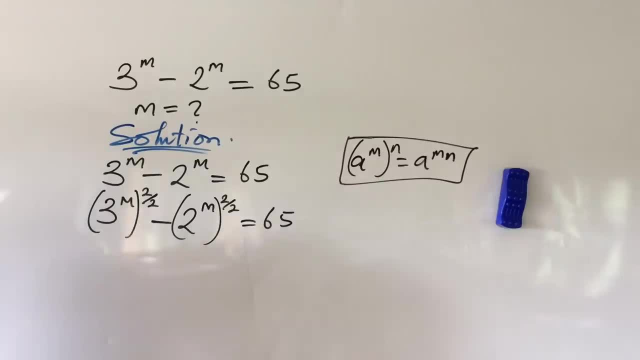 occasions. okay. so if we suck up to this slope, we can bring in this fraction. yeah, we can bring in this fresh or year also, and so we can rewrite this as your: 3 to the power of your m all over 2. close bracket: all to the power of 2 minus. same thing. we have here m all over 2. 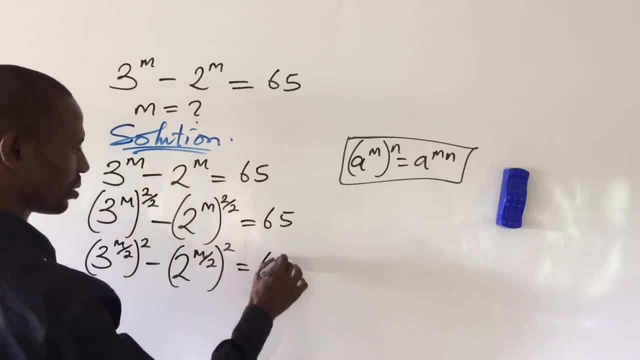 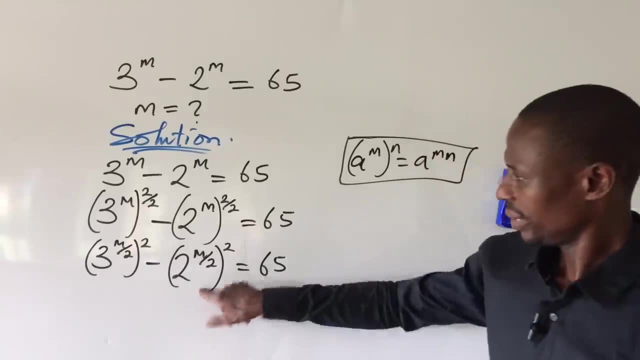 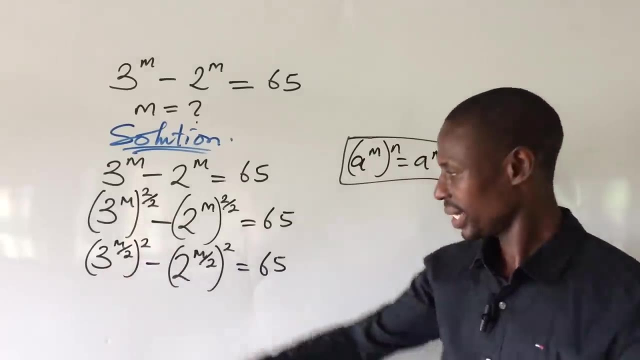 all to the power of 2, equal to 65. easy, okay, so we now have a square. we have a square so we can bring in different letters to represent what we have in the bracket here and what we have in the bracket here, because what we have in here and here are different, so we are giving bringing. 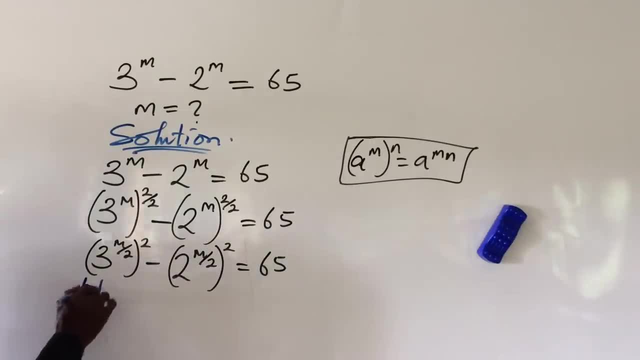 different letters. so we cannot say here, let's- um, let's take x be equal to our 3 to the power of m all over 2. then we have take the second one, y, equal to 2 to the power of m all over 2. okay, so. 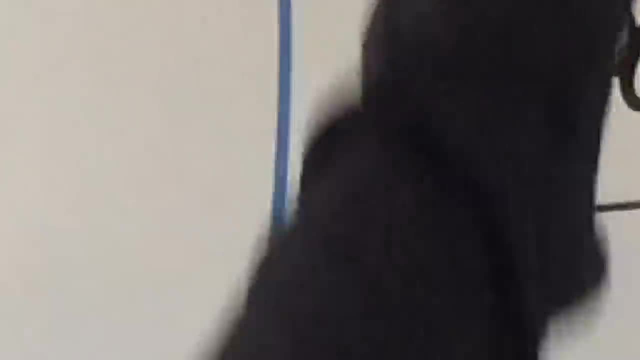 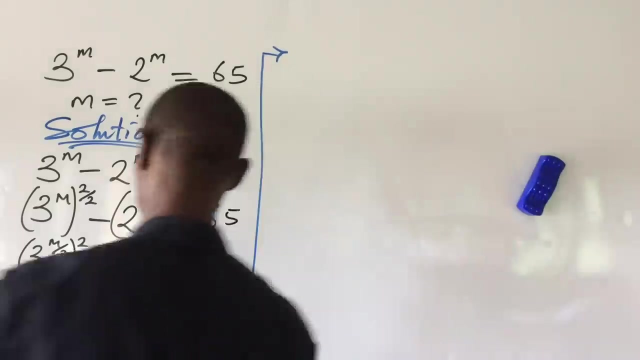 let's proceed from here. so let's go ahead and pull, pull, pull this x into here and y into this position, this x into here and y into this position, this x into here and y into this position. so if we do that, we're going to have this to be. 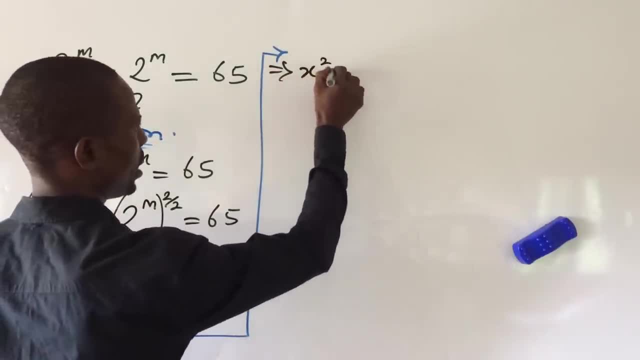 so if we do that, we're going to have this to be so. if we do that, we're going to have this to be your. this now implies our x squared minus your. this now implies our x squared minus your. this now implies our x squared minus y squared equal to. 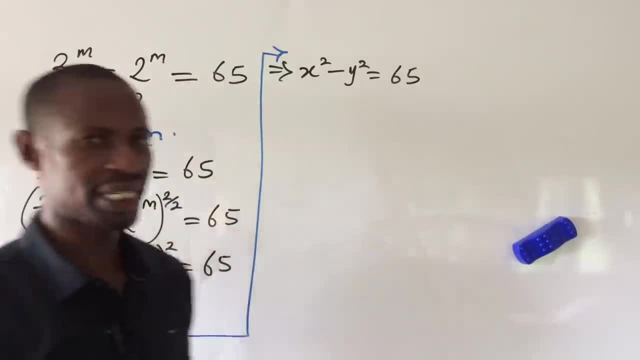 y squared equal to y squared equal to 65.. 65.. 65.. the game is playing out now. all right, the game is playing out now. all right, the game is playing out now. all right, now, let's look at this again. now, let's look at this again. 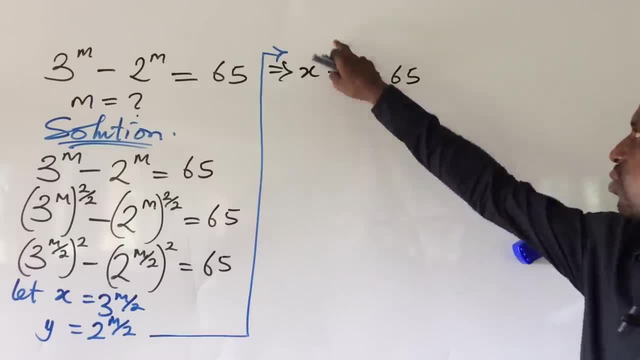 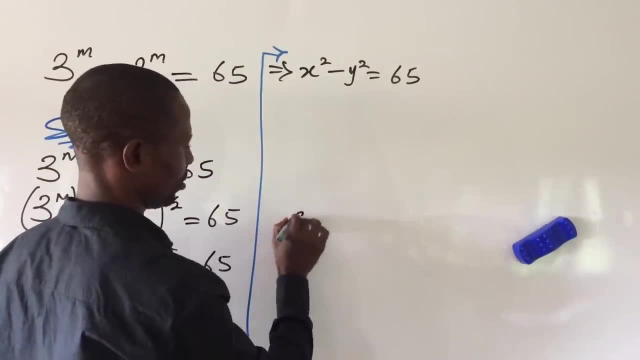 now let's look at this again. yeah, we can apply the difference of two. yeah, we can apply the difference of two. yeah, we can apply the difference of two square because they are having a square minus y squared. so the difference of two squares is that if you have um, your a squared minus b. 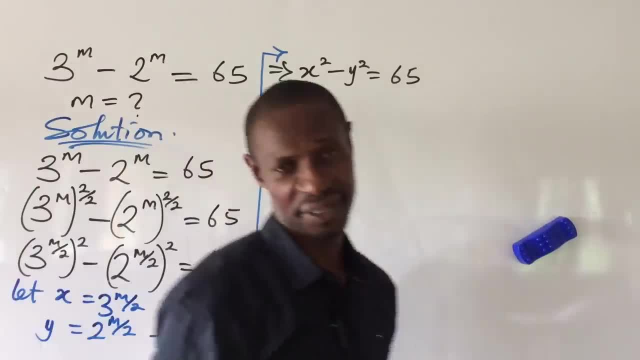 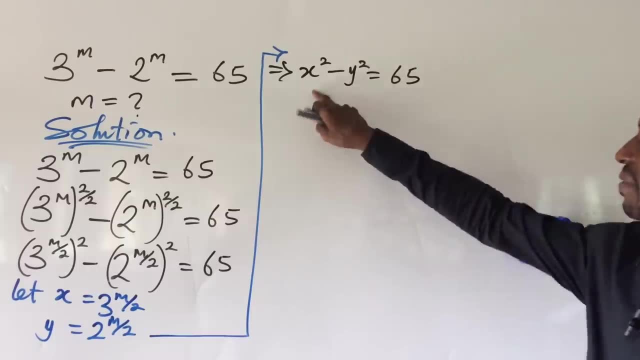 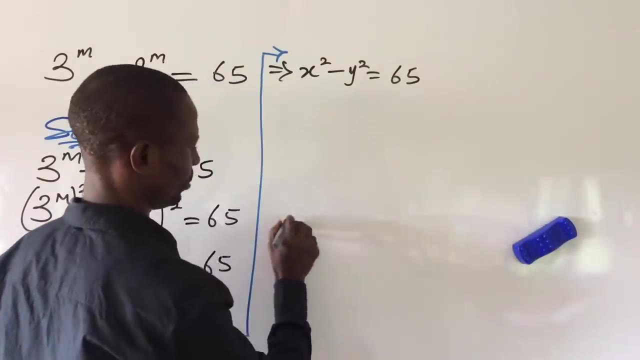 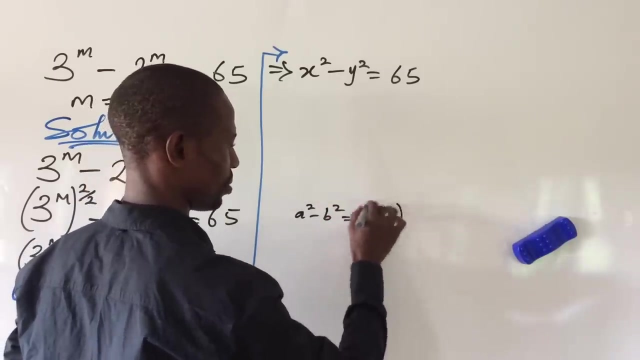 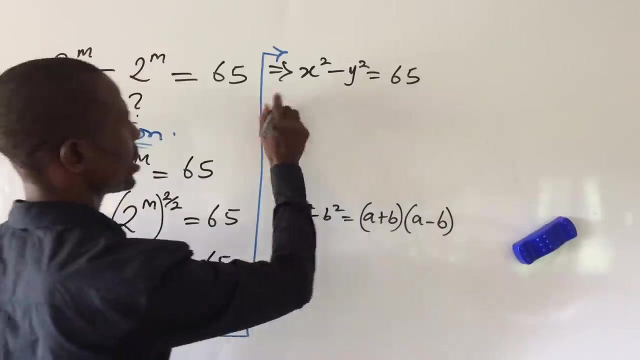 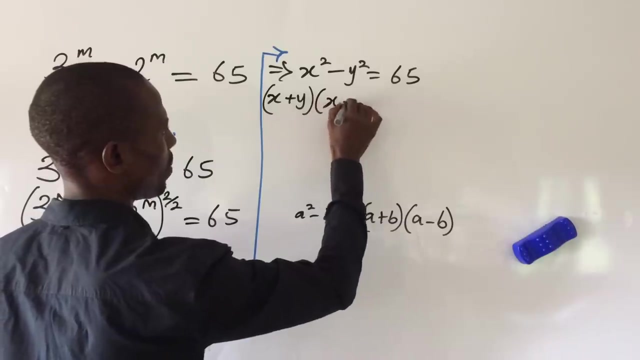 the game is playing out now. all right, now let's look at this again. here we can apply the difference of 2 squared because they are having x squared minus y squared. here we can apply the difference of 2 squared because they are having x squared minus y squared. so the difference of 2 squared says that if you have um your a squared minus b squared, this is equal to a plus b plus bracket bracket, a minus b. so if we succumb to this rule, then we can rewrite this as our x plus y close bracket. then bracket your x minus y close bracket are equal to 65.. here we can apply the difference of 2 squared because they are having x squared minus y squared. so the difference of 2 squared says that if you have um your a squared minus b squared, this is equal to a plus b close bracket bracket a minus b. so if we succumb to this rule then we can rewrite this as our x plus y close bracket. then bracket your x minus y close bracket are equal to 65.. 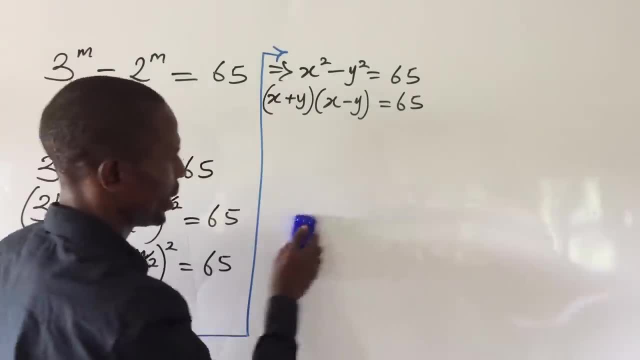 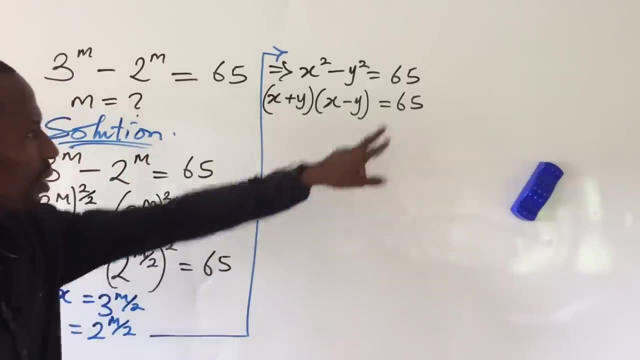 here we can apply the difference of 2 squared, because they are having x squared minus b squared. this is equal to 65.. good, let's take down this again now. if you look at this expression here, now we can subscribe to this product rule, okay, but here we must get two numbers from here that we can equate these two. 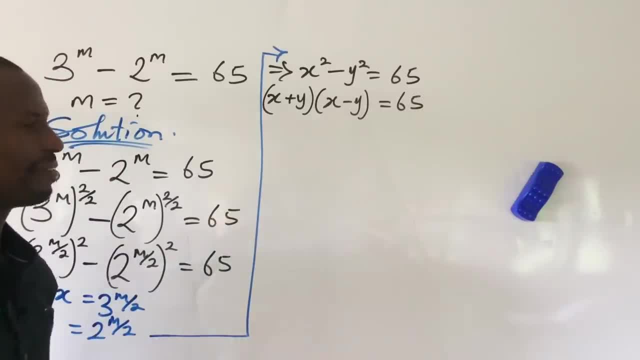 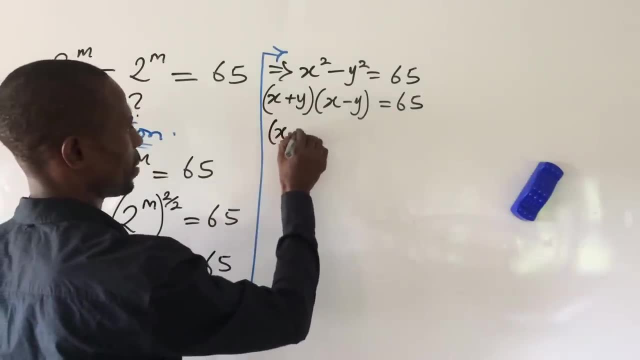 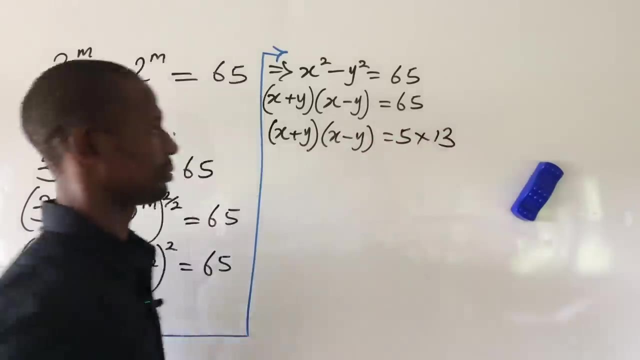 and so we look at 65. we can rewrite 65 as 5 times 13 and so this winner becomes: bracket your x plus y r into x minus y, equal to 5 times 30. we can equate this to the first time here. equate this to this. but if you 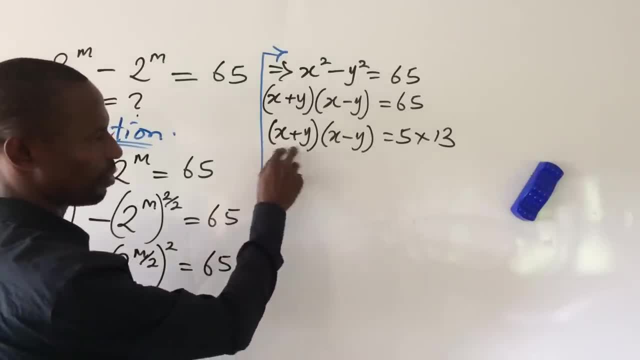 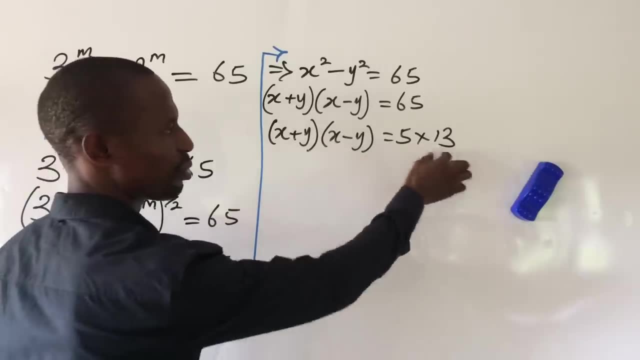 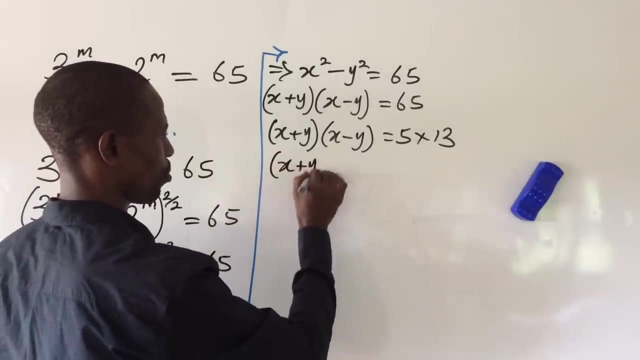 take a look at this: here we are having a plus, so the sum of these two numbers must be greater than the subtraction of this two number, and so we have to rewrite the expression we have on the right hand side. so our expression will now becomes your x plus y bracket, x minus y, equal to 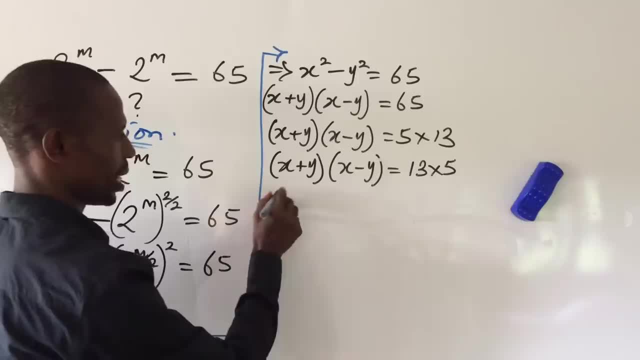 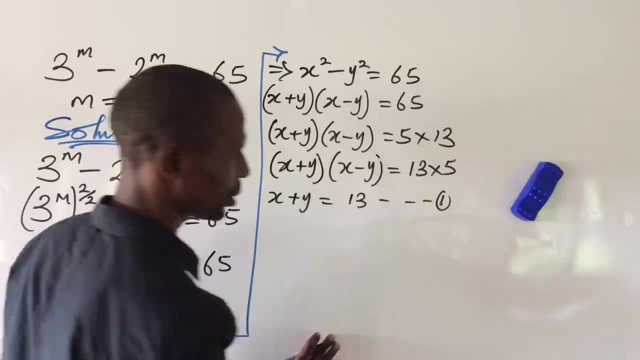 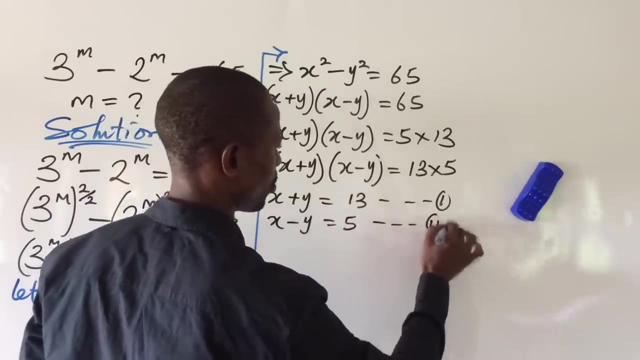 13 times 5.. with that, this now implies that x plus y equal to your 13. let's take this as the equation one. then your x unminus y equal to 5.. let's take this as our equation two. now, if you look at this two equation automatically, this is the simultaneous equation, so we can solve these. 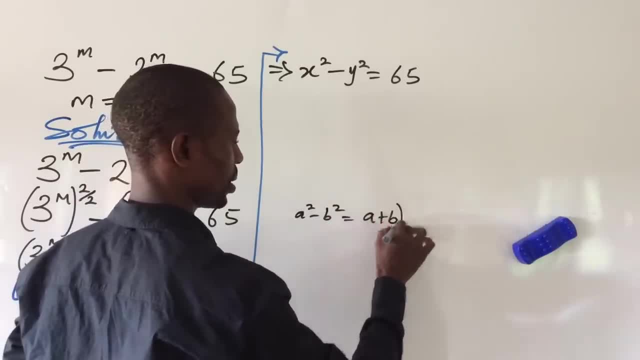 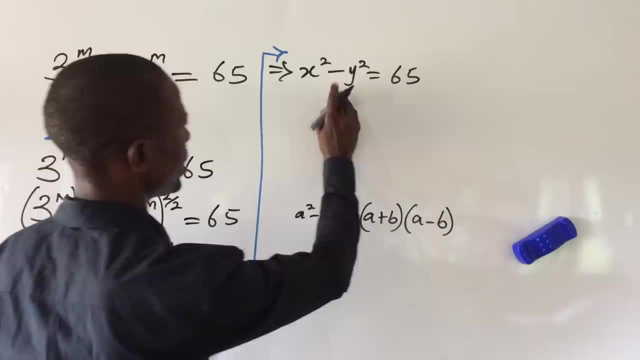 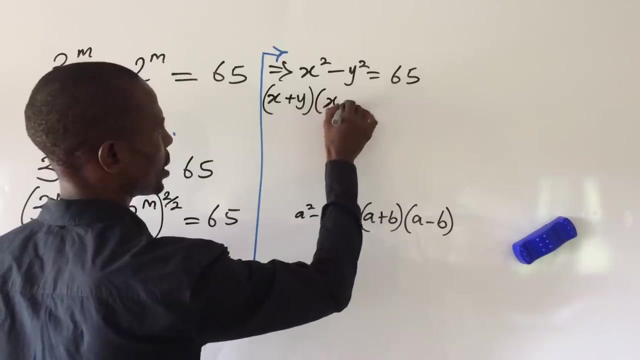 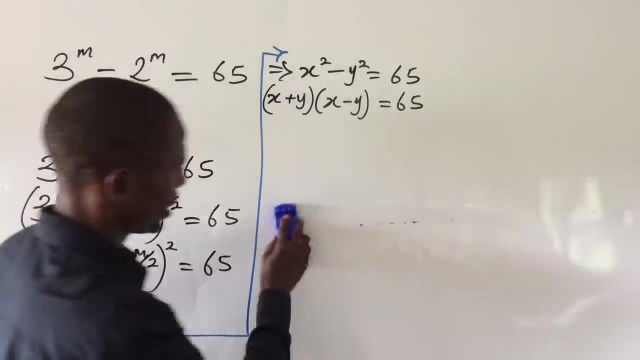 squared, this is equal to a plus b plus bracket bracket, a minus b. so if we succumb to this rule, then we can rewrite this as our x plus y plus bracket. then bracket, your x minus y plus bracket are equal to 65.. good, let's take down this again now. if you look at this expression, 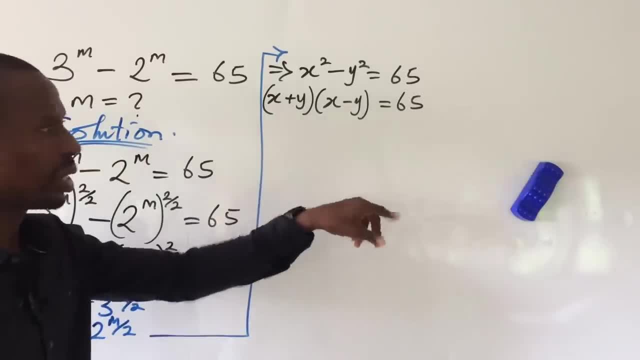 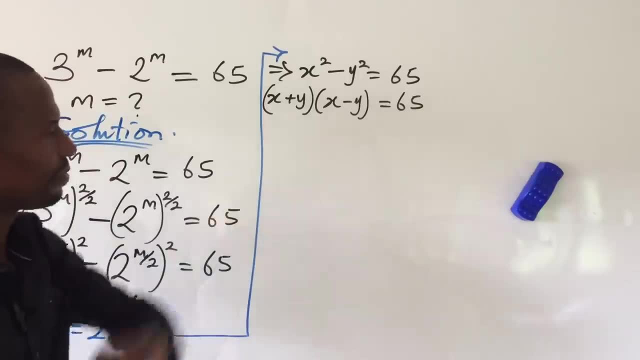 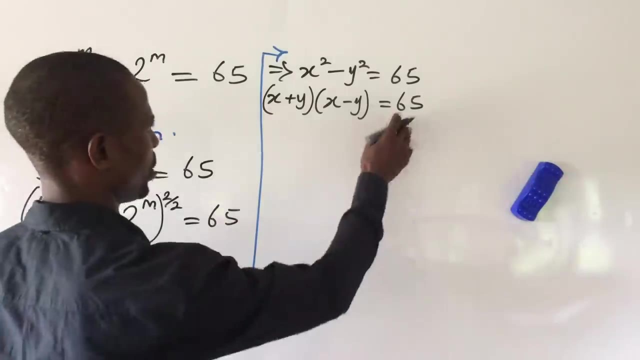 here. now we can subscribe to this product rule, okay, but here we must get two numbers from here that we can equate these two. and so we look at 65. we can rewrite 65 as 5 times 13, and so this will now becomes bracket, your x plus y. 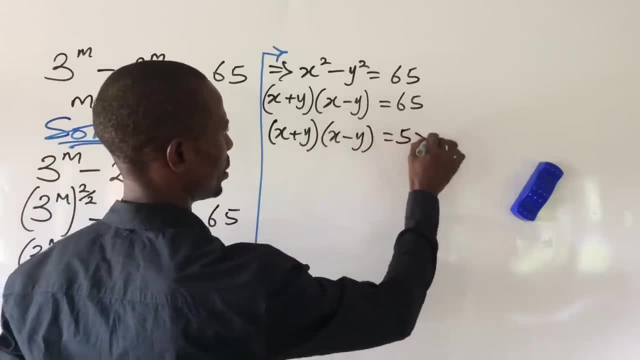 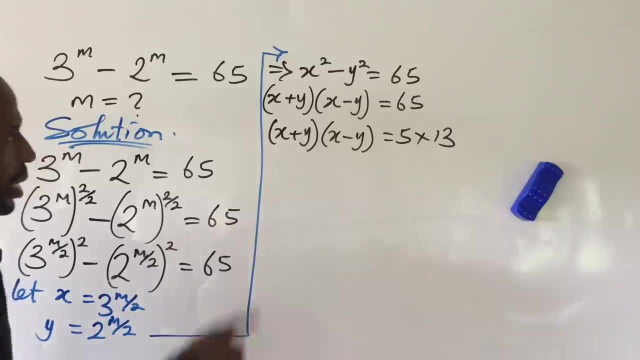 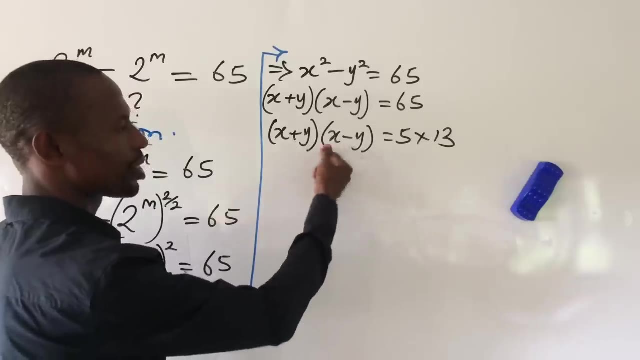 r into x minus y, equal to 5 times 30.. we can equate this to the first time here, equate this to this. but if you take a look at this here we are having a plus. so the sum of these two numbers must be greater than the subtraction of this two number, and so we have to rewrite the expression. 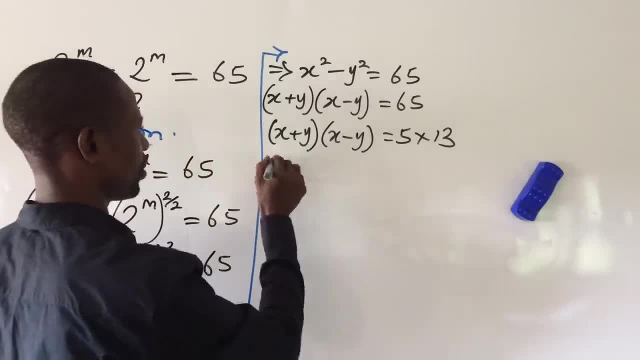 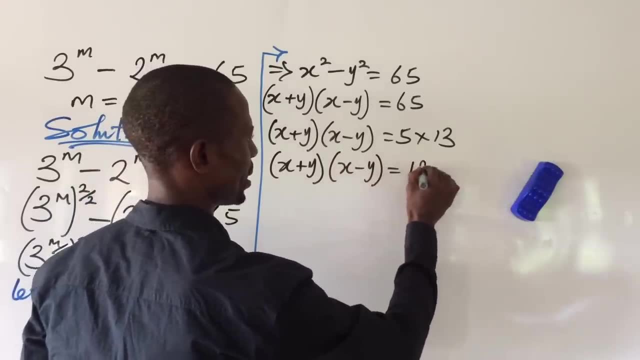 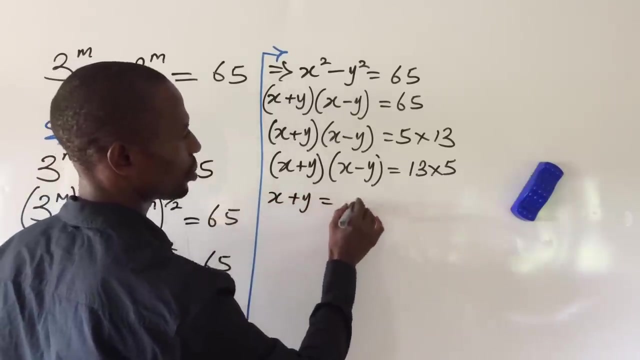 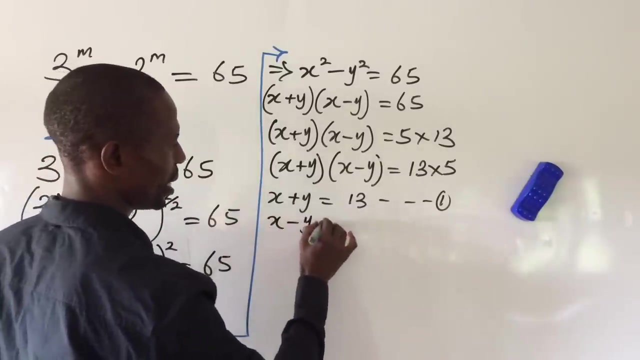 we have on the right hand side. so our expression will now becomes: your x plus y bracket- x plus y minus y equal to 13 times 5.. with that, this now implies that x plus y equal to your 13. let's take this as the equation 1. then your x minus y equal to 5. let's take this as our equation. 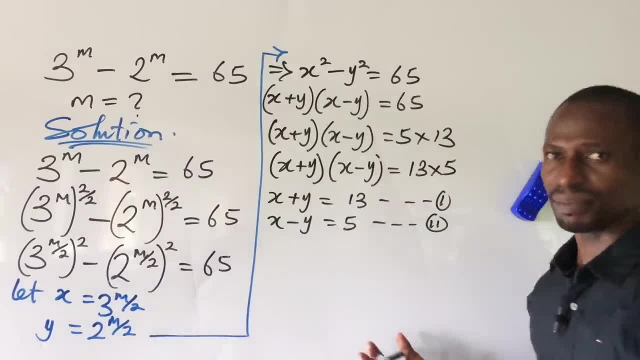 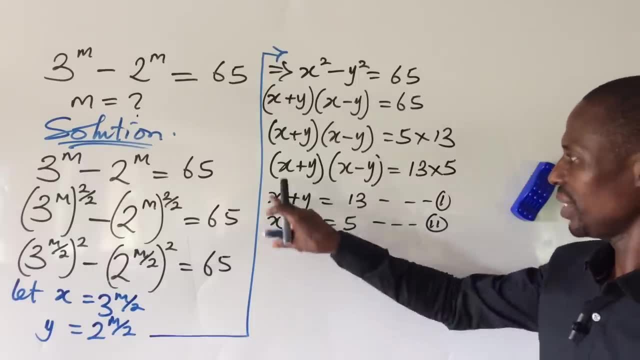 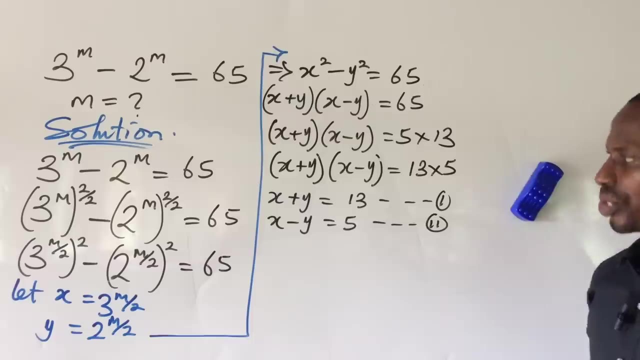 2. now, if you look at these two equations automatically, this is a simultaneous equation, so we can solve these two equations simultaneously. how do we go about this? now we're having x here, x. here, the coefficient is 1, 1, y here, y- here, the coefficient is 1: 1. 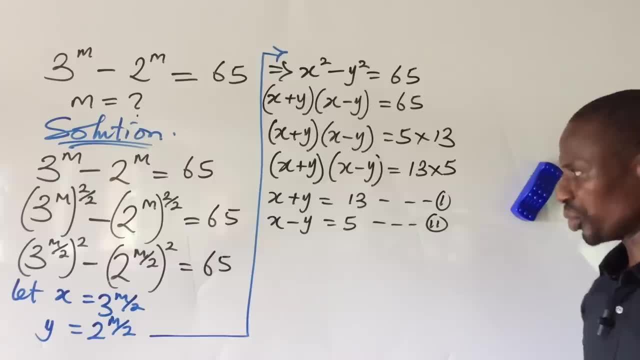 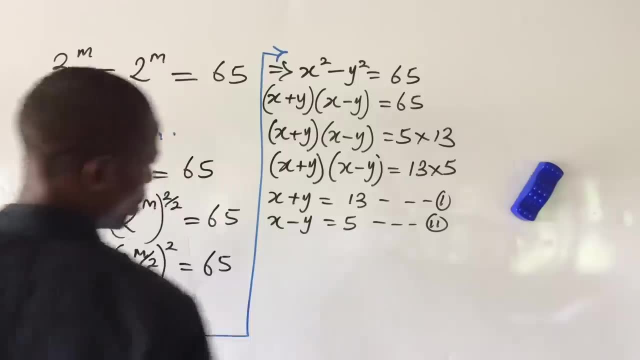 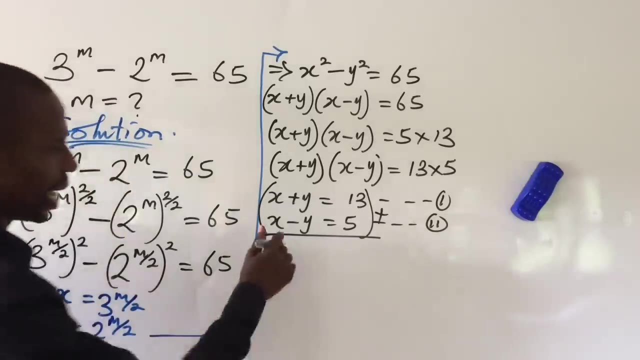 so we can either add or subtract equation 1 from 2.. but because we're having plus and minus here, so we're going to add equation 1 to equation 2.. so if we go ahead to add equation 1 and 2, so let's put this: we're adding. so if we add this, automatically, plus y, minus y will leave the system. 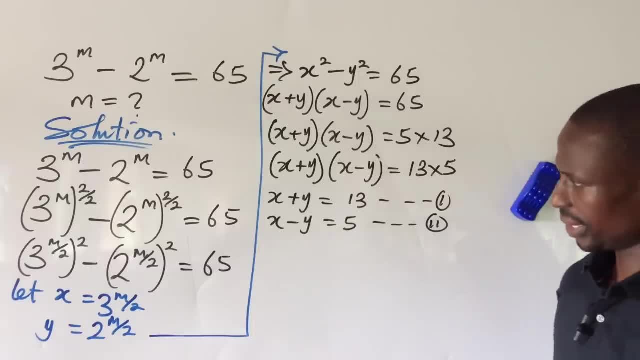 two equations simultaneously. how do we do about the x? now we're having x. everything in the second column we have x subtracted. so the number of cycles left in the thatviolet is equal to the number of times up by 5. n over x plus y equals 2.. urious вкус japon. we can solve these two equations simultaneously. basically, how do we do about x? now we're having x in the second column, which we have. its integration with the theca lasciar in the second column is the same as this and vice versa. now we NW. 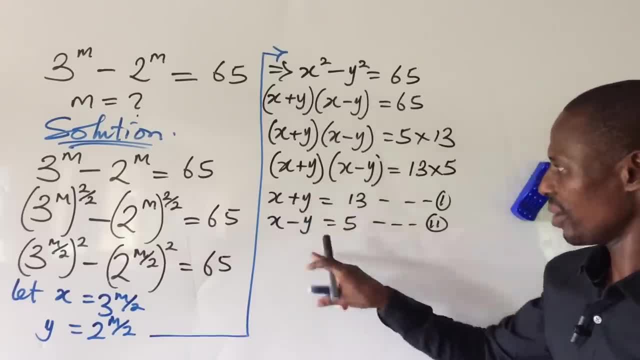 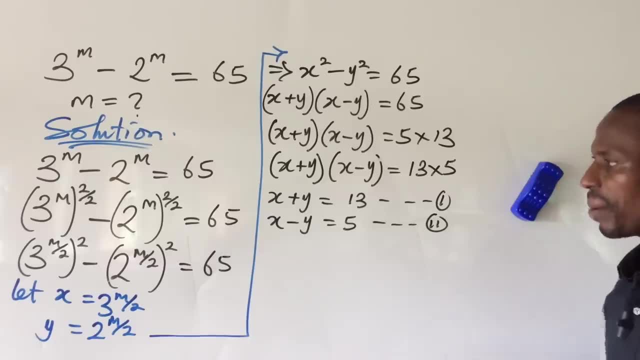 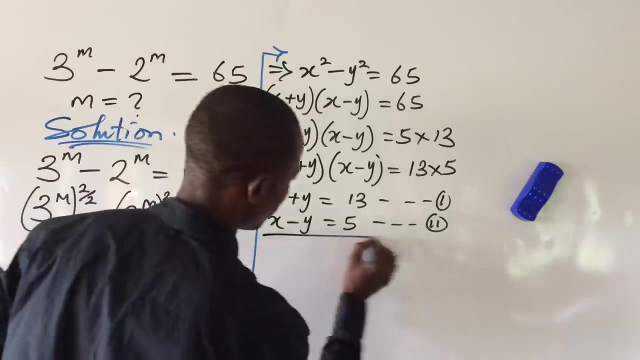 x- here the coefficient is one one. y here: y- here the coefficient is one one. so we can either add or subtract equation one from two. but because we're having plus and minus here, so we're going to add equation one to equation two. so if we go ahead to add equation one and two, so let's put: 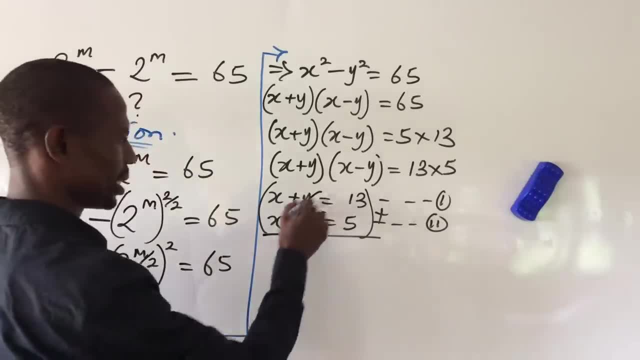 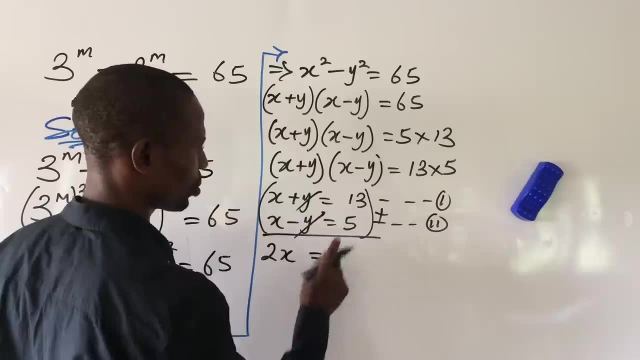 this we're adding. so if we add this automatically- plus y, minus y- we leave the system. we give our zero, so we're left with 2x equal to 13 plus 5. we give us here 18 divided by 2, then this will give. 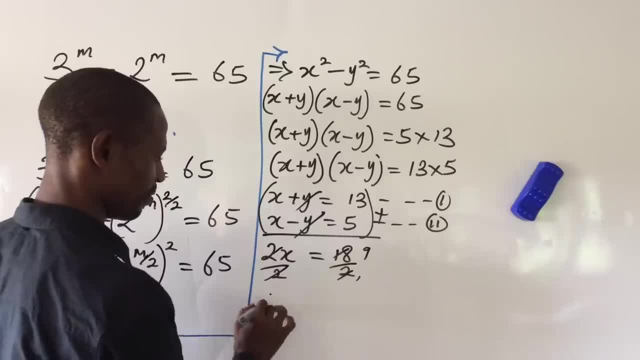 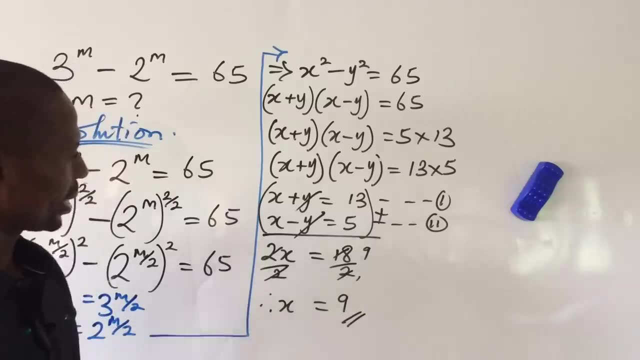 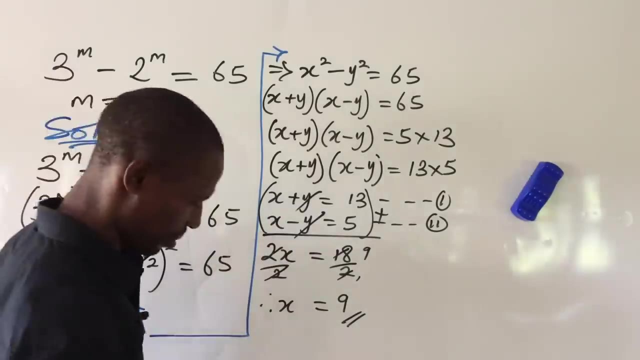 us. here one one and here one. here we have nine, so we have. therefore, rx is equal to nine. easy, we've gotten our x, so let's go ahead and get our y. we can put y into either of the equation, but let's take um equation one, okay, so from here we'll say put. we'll say put. 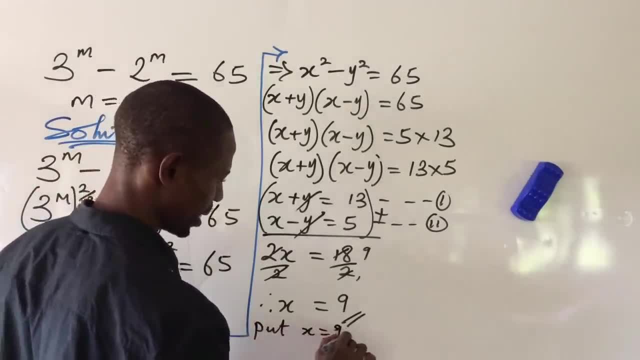 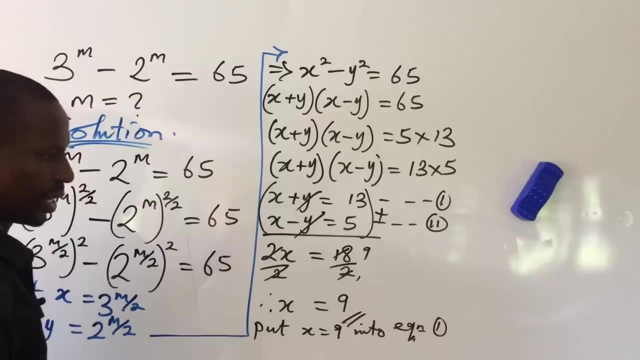 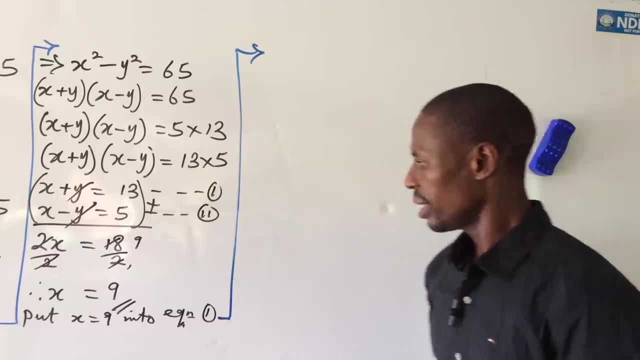 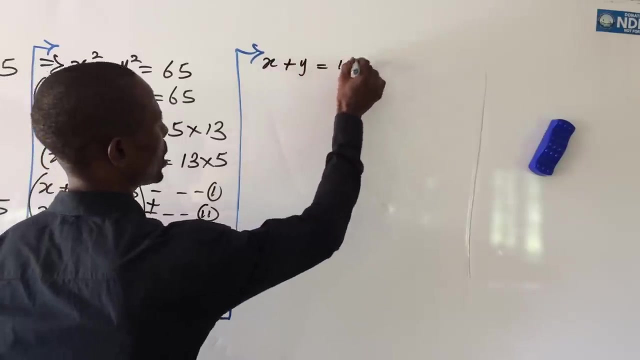 okay, put x equal to 9 into equation, into equation one. look at our equation one. yeah, so let's proceed again from here. okay, what does that mean whenever we see x? let's put in um my day and just simplify. so our equation one is your x plus y equal to 13. so here we have 9 plus y equal to 13, y equal to. 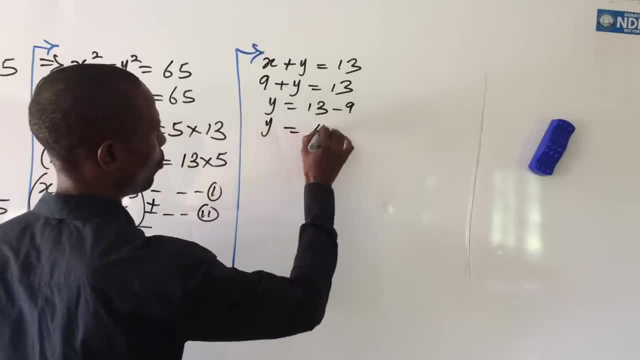 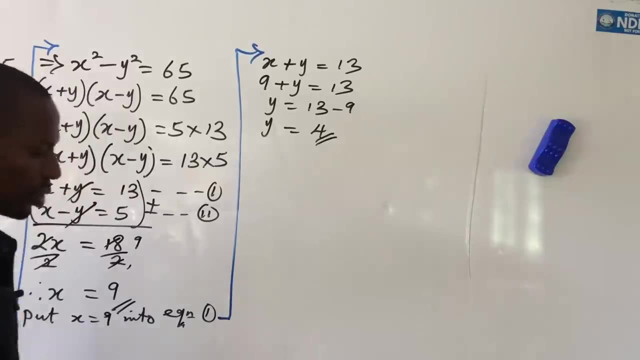 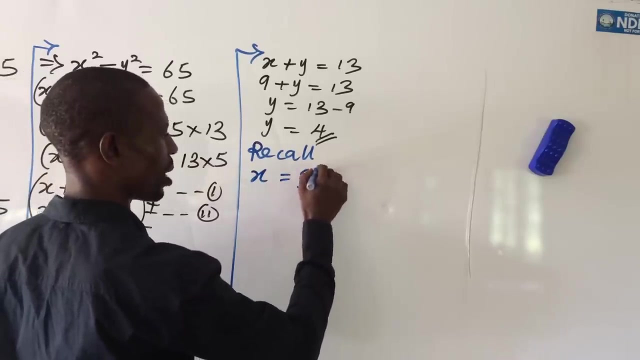 14 minus 9, therefore y equal to 4.. simple as abc. but recall, uh, just a place where we said: let your x be equal to. so from here we will now recall. recall where we said: uh, let x be equal to 3 to the power. 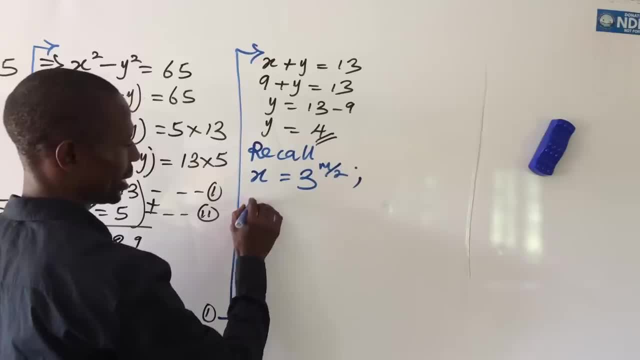 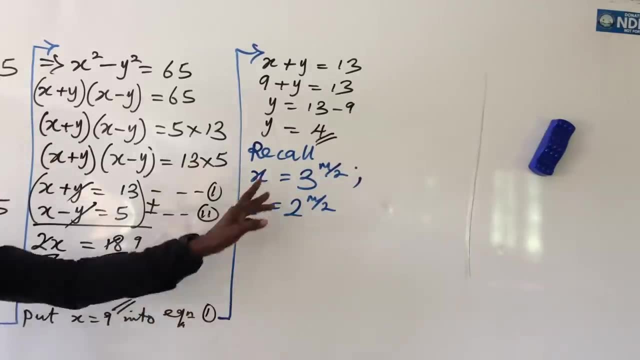 of m all over 2 and y equal to your 2 to the power of m all over 2. so we succeeded in getting this two numbers now. so we succeeded in getting these two numbers now. so we want to get the value of our m from here. so let's take the first one, the first one. 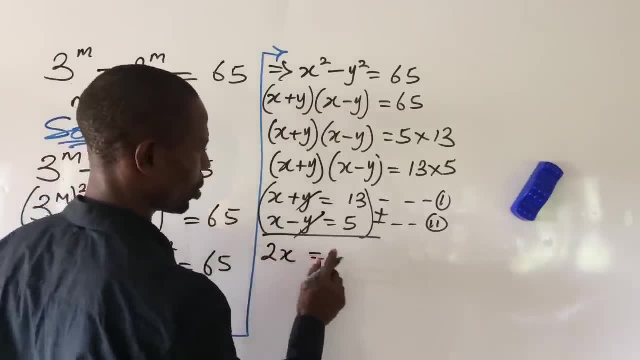 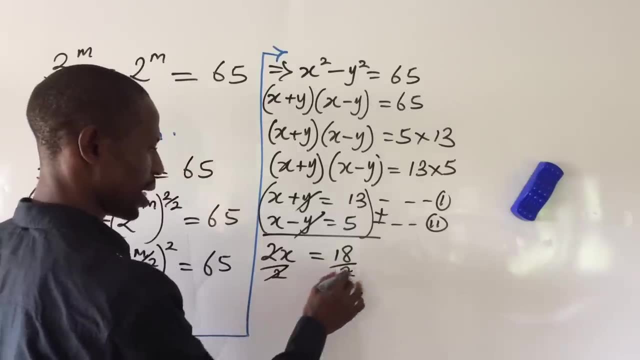 we give us 0, so we're left with 2 x equal to 13 plus 5. we give us here 18 divided by 2, then this will give us here 1, 1 and here 1. here we have 9, so we have. therefore our x is equal to 9.. 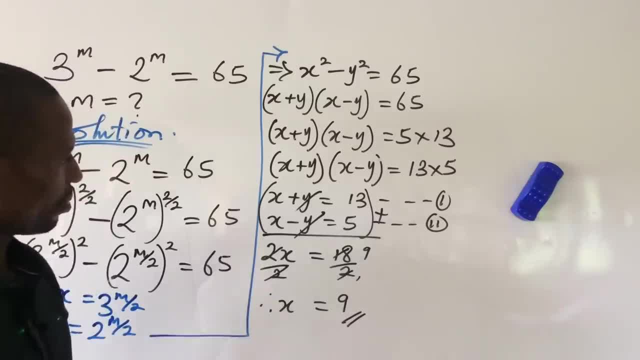 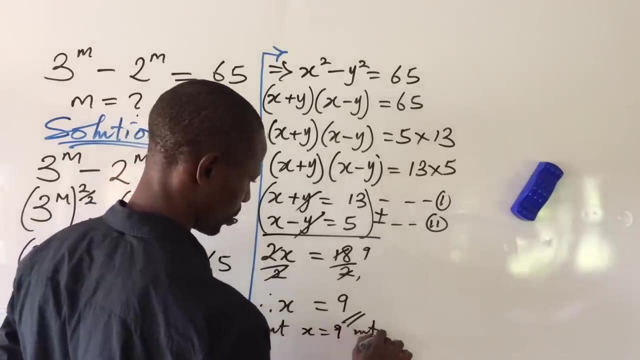 easy. we've gotten our x, so let's go ahead and get our y. we can put y into either of the equation, but let's take um equation one, okay, so from here we'll say put. we'll say, put, put x equal to 9 into equation, into equation one. look at our equation one. yeah, 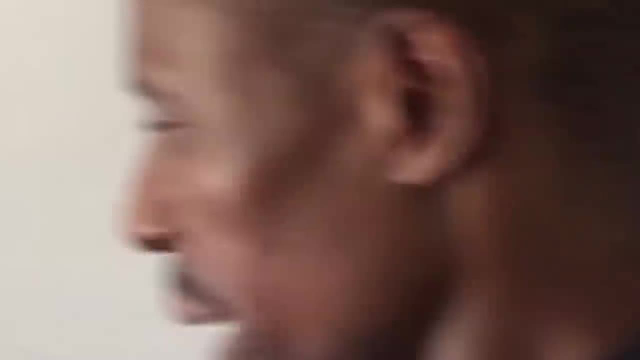 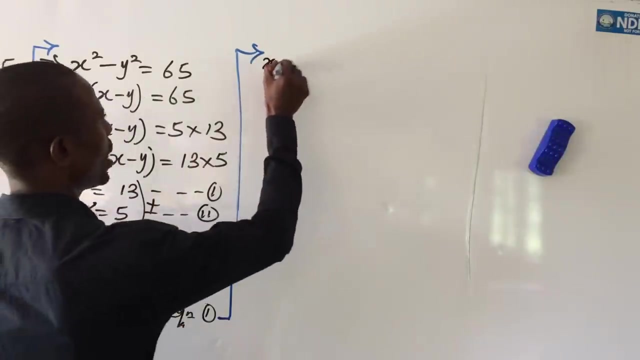 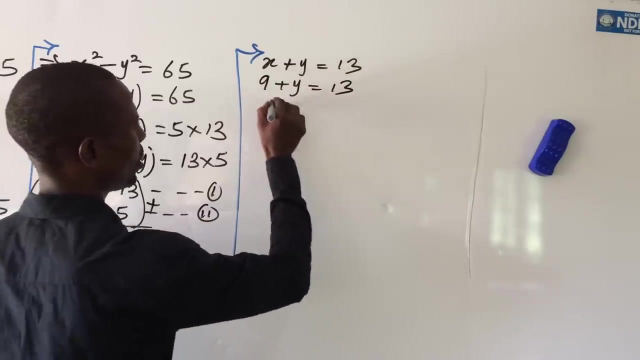 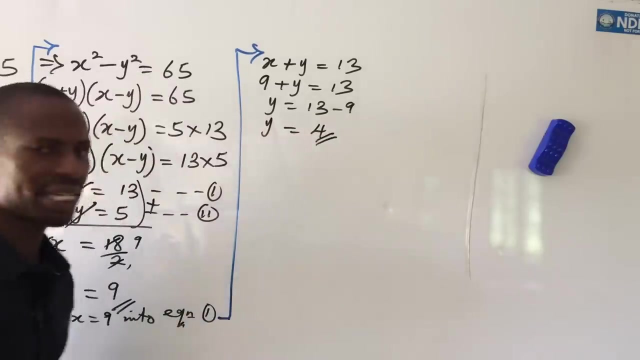 so let's proceed again from here. okay, what does that mean? whenever we see x, let's put in um nine there and just simplify. so our equation one is: your x plus y equal to 13.. so here we have 9 plus y equal to 13. y equals to 13 minus 9, therefore y equal to 4.. simple as a, b, c. but to 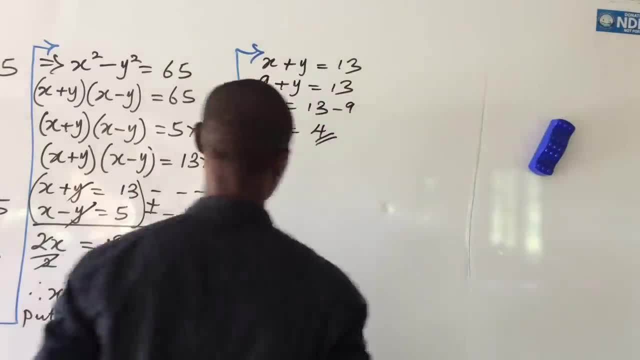 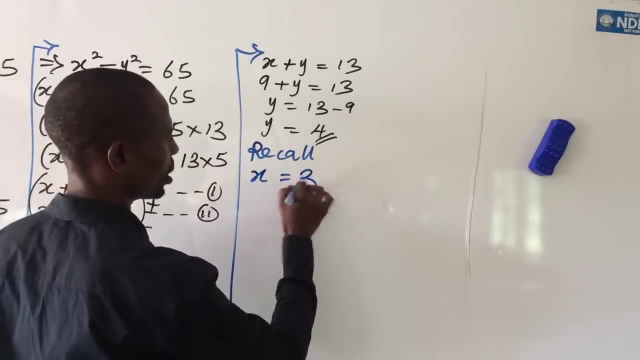 recall: uh, there's a place where we said: let your x be equal to so from here we now recall. recall where we said: uh, let x be equal to 3 to the power of m all over 2, and y equal to your 2 to the power. 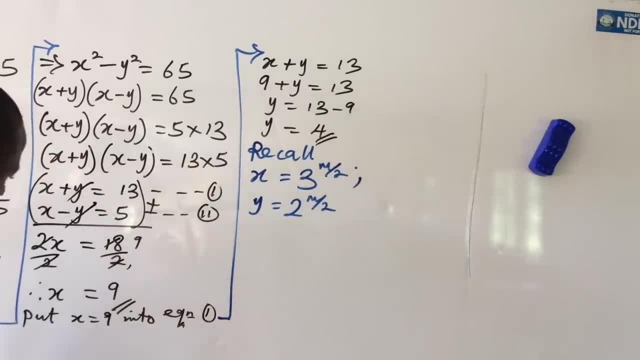 of m all over 2.. so we succeeded in getting these two numbers now. so we want to get the value of our m from here. so let's take the first one. the first one. we have case one where we have our x equal to 9.. so, looking at this, 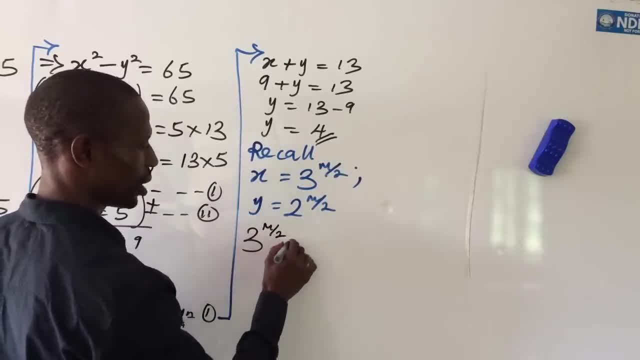 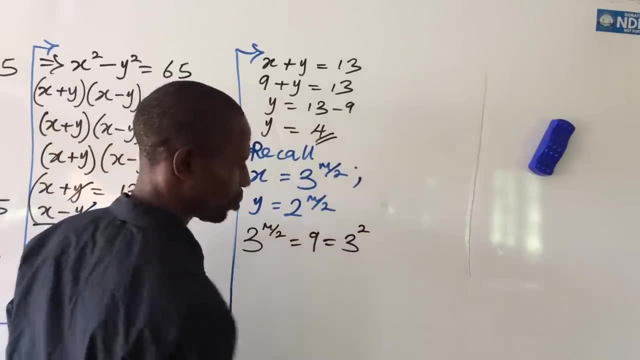 will now give us 3 to the power of m all over 2 equal to 9.. we are having base 3 here, so we can equally express 9 as 3 to the power of 2.. okay, so the bases are now the same, and so this: 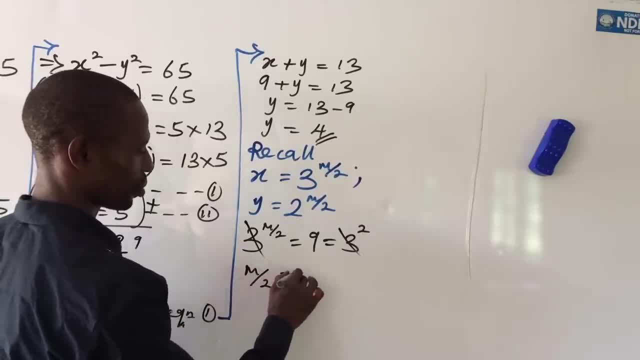 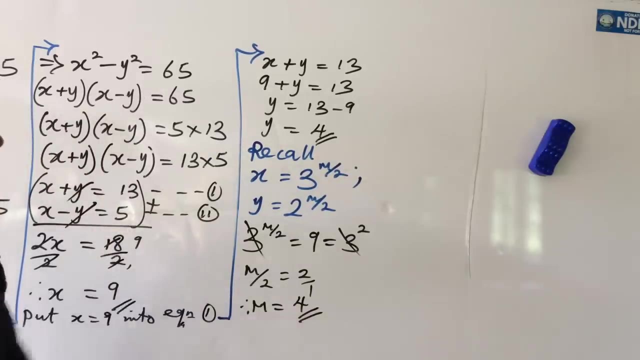 we go with this. when i have m all over 2, equal to 2. this is all over every single one. so if we cross multiply, then this will not give us. therefore, m is equal to your 4. this is the value for our m. now, if we go ahead to a substitute 4 for y into this expression here, 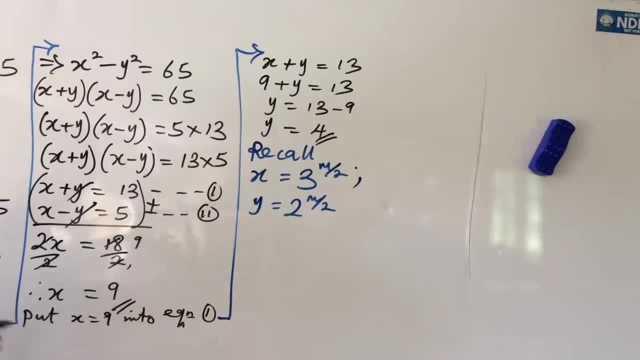 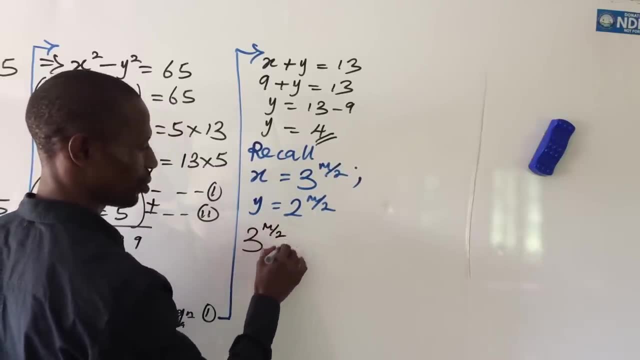 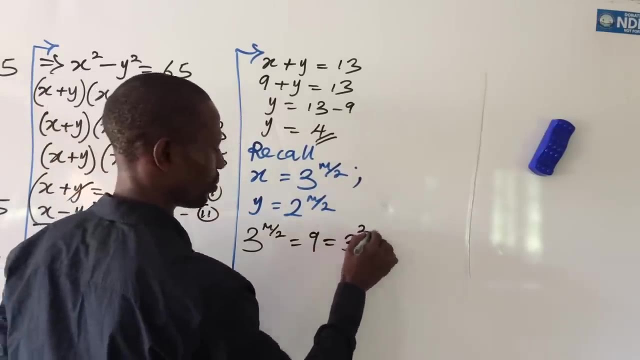 we have case one where we have our x equal to um nine. so, looking at this, this will now give us three to the power of m, all about two equal to nine. we are having base three here, so we can equally express nine as three for the power of two. okay, so the bases are not the same, and so 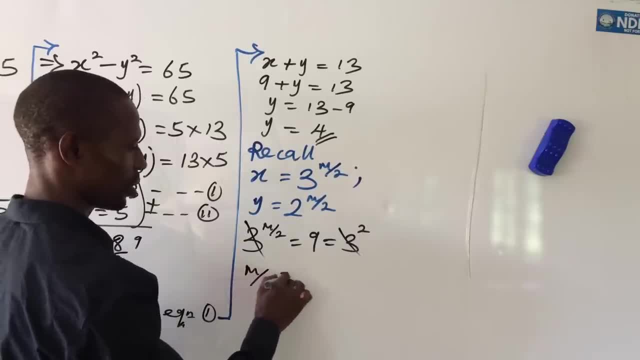 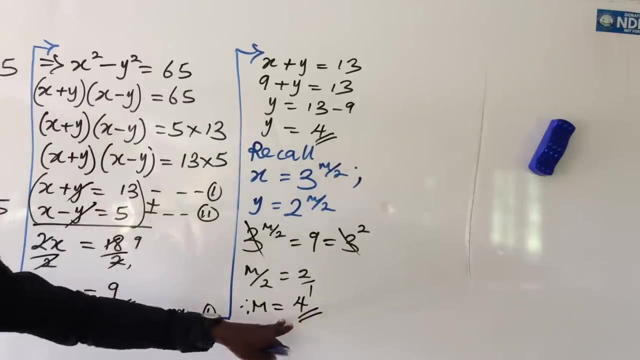 this. we go with this when i have m all over two equal to two, this all over visible one. so if we cross multiply, then this will not give us. therefore, m is equal to your four. this is the value for our m. now, if we go ahead to a substitute four for y into this expression here, we are still going to. 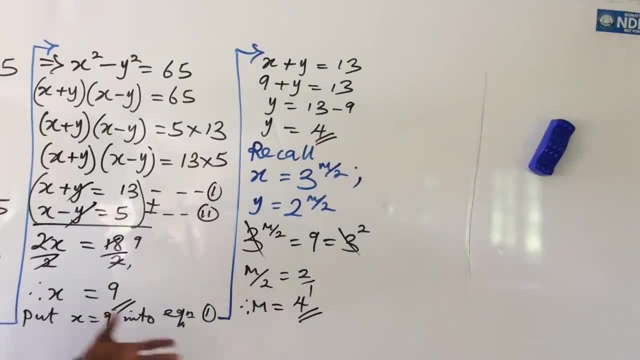 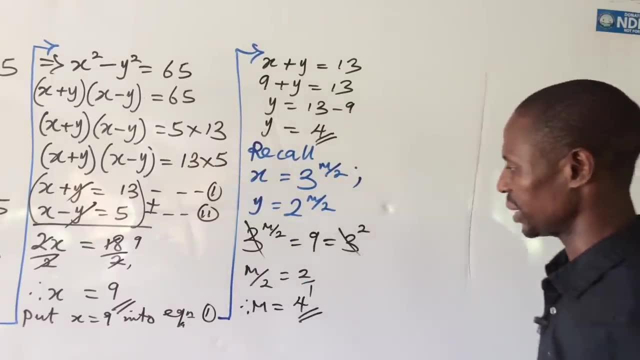 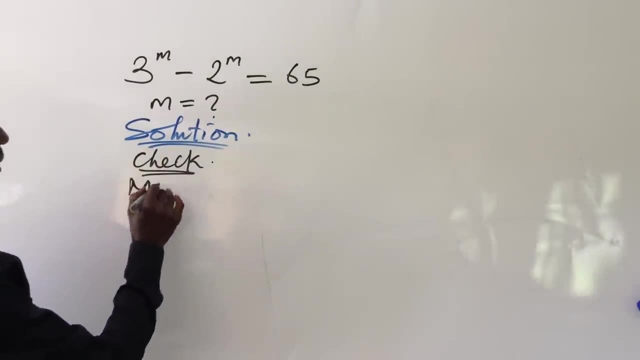 get the value of m to be four. but what we want to do here is this: we want to check if the value m correspond always satisfy our equation. so, yeah, we want to check. all right, so we want to check here. now, okay, that we solve our m equal to four. so let's bring. 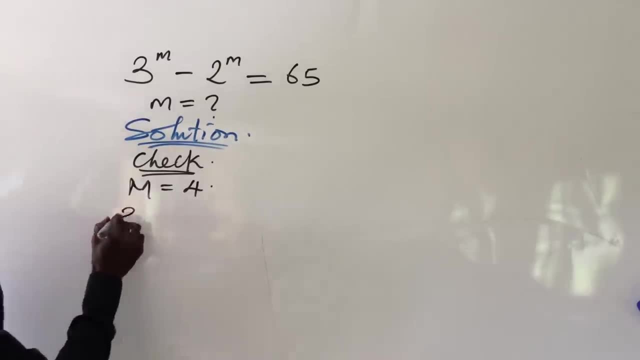 down the question wherever we see, and let's put in further. so this will give us three to the power of four, a minus two to the power of four, equal to 65. what is three to the power of four? that is three, and that will give us what? 81. okay, then, minus two to the power of four means two times two times two. 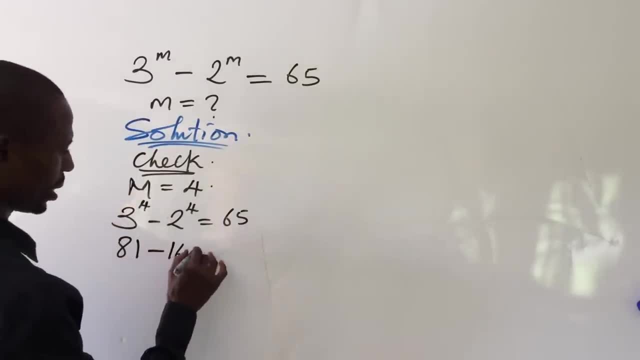 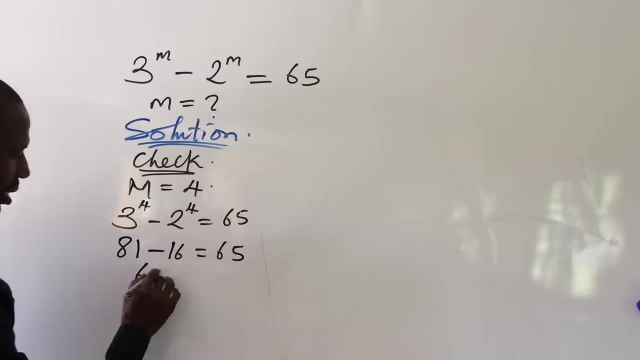 times two, that will give us um 16- okay, equal to 65. then 16 from um h1 will give us what? 65, which is equal to 65. so this shows that the value of m we should suffer to be um four is what called red. 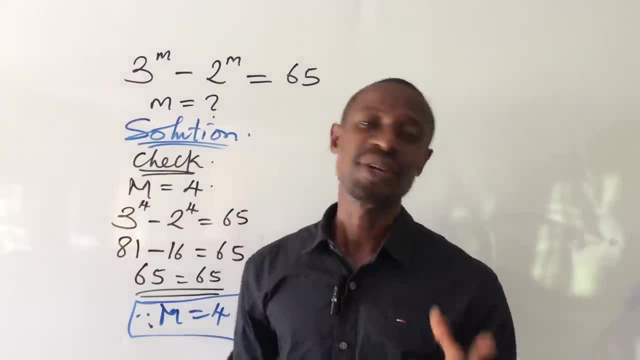 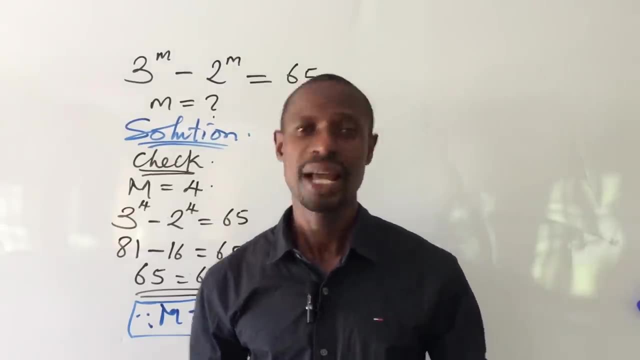 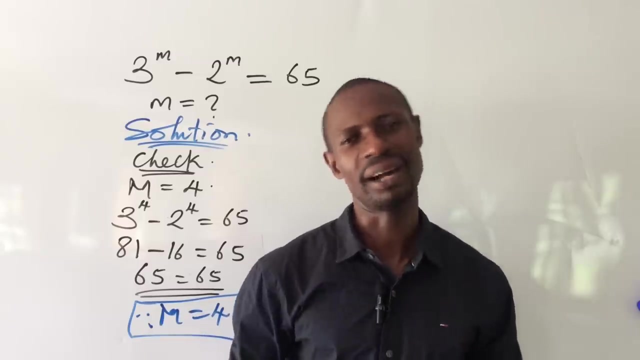 q, e, d, so so if you learn something from this math- only paired a question, the solution to this math- only paired uh question, then drop it in the comment section. if you love what is going on here, do not forget, do not hesitate to share with family or friend members who need this our knowledge of.